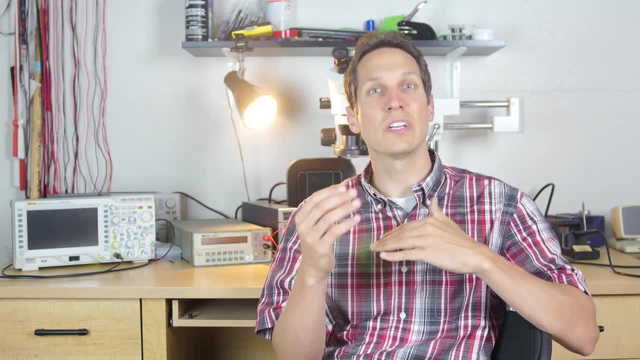 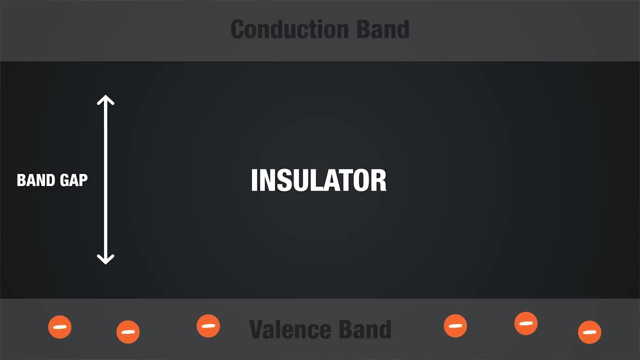 diagram of three types of materials used in electronics and discuss the conductivity of each material based on their bandgap. As we can see, the bandgap between the valence band and conduction band in an insulator is really big. This is why it doesn't conduct current. The bandgap in a semiconductor is: 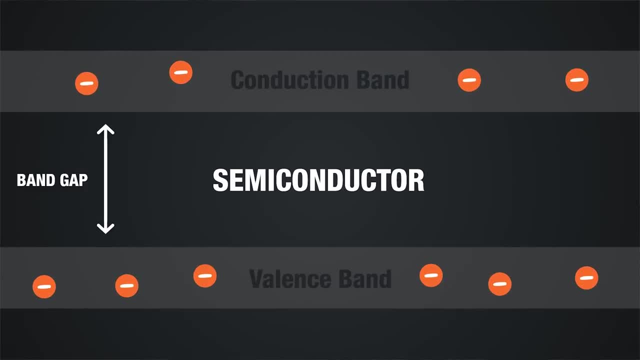 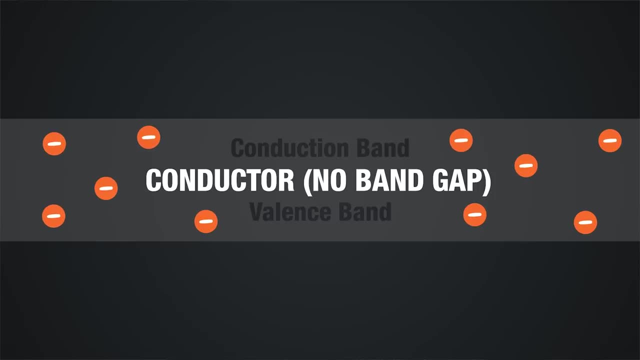 smaller compared to an insulator and allows a valence electron in the valence band to jump into the conduction band if it receives external energy. In a conductor like copper there is no bandgap. Actually, the conduction band and valence band overlap, which means 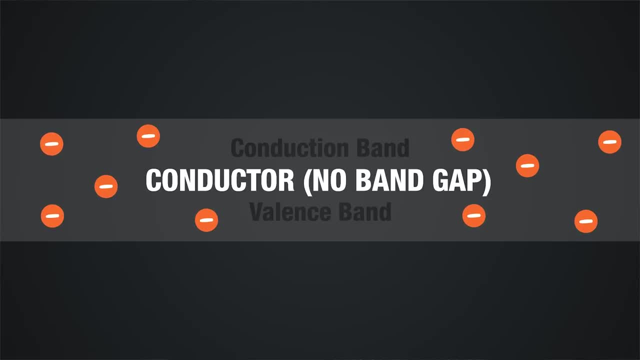 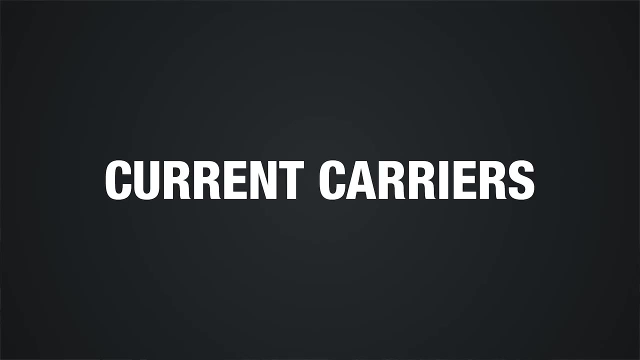 the electrons can freely move into the conduction band. This is why you may hear the electrons in metal referred to as a sea of electrons. They're just floating around. Now that we know more about bandgap, let's discuss the two types of current carriers. 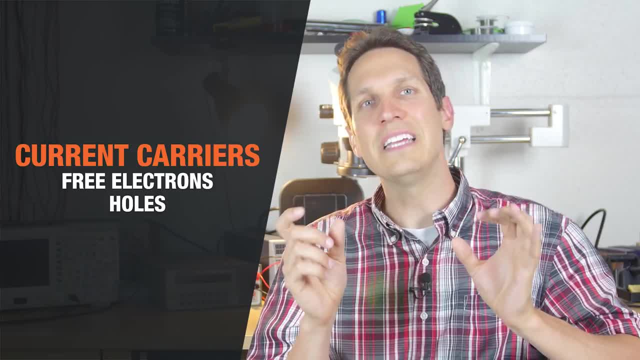 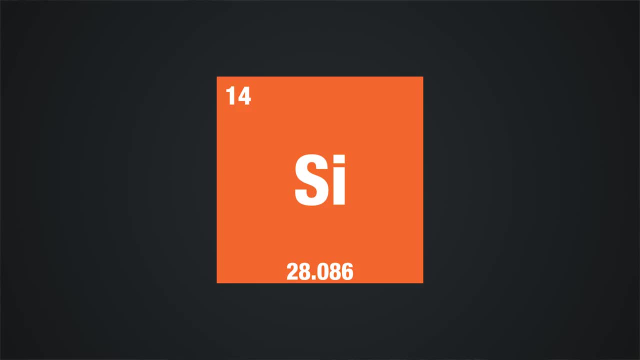 in a semiconductor, free electrons and holes and see how they produce currents. in a semiconductor, Atoms may combine to form a solid crystalline material through covalent bonding. For example, a silicon atom covalently bonds with four adjacent silicon atoms to form an intrinsic. 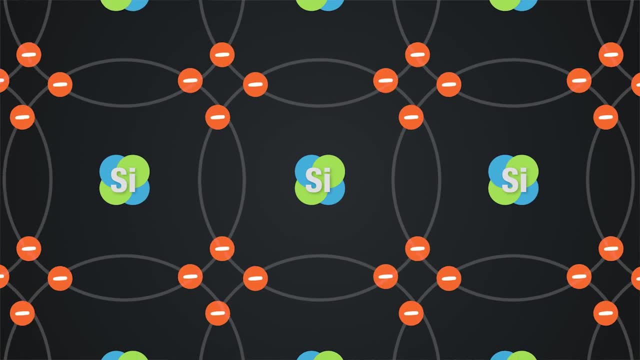 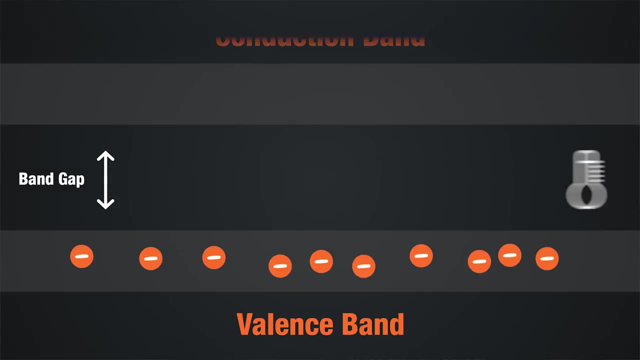 silicon crystal: Intrinsic because it doesn't contain impurities, and a crystal because there is a pattern in how the atoms are connected In a capacitor. intrinsic silicon crystal gains enough heat energy that enables some of the valence electrons to jump into the conduction band, becoming free electrons. 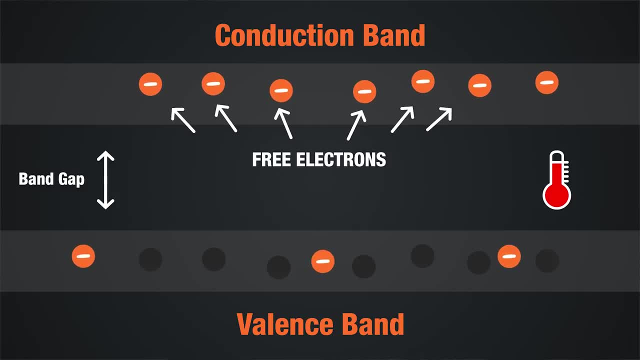 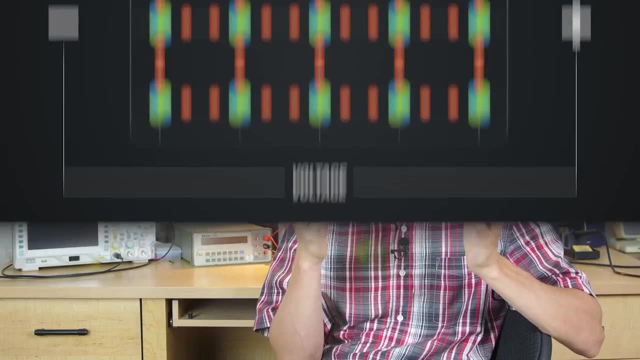 When this happens, vacancies are left in the valence band within the crystal. These vacancies are known as holes. If we put a voltage source across an intrinsic silicon material, the thermally generated free electrons in the conduction band will be attracted to the positive. 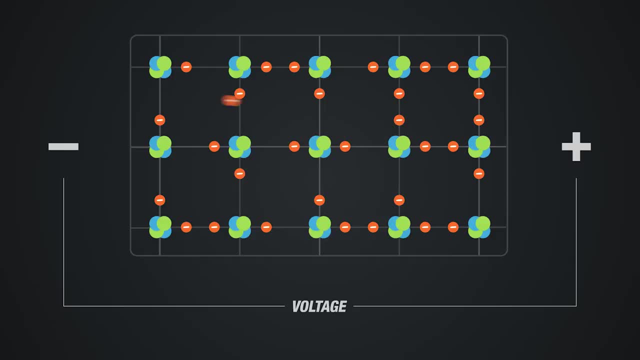 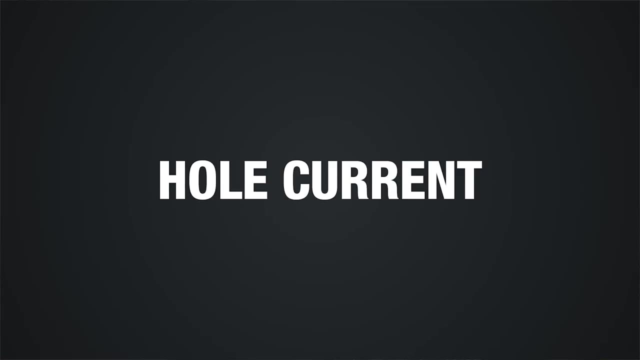 end of the voltage source, They will move towards the positive end and this movement produces current in the material. This type of current is called electron current. While electron current happens in the conduction band, the other type of current, hole current, 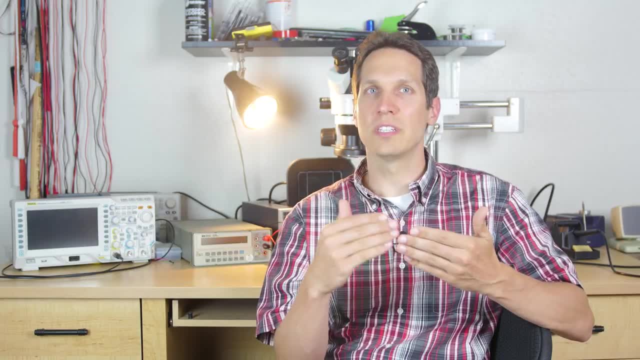 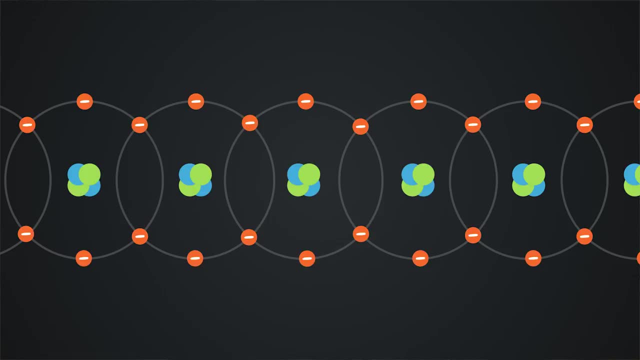 happens in the valence band. Remember that as valence electrons jumped into the conduction band, vacancies or holes are left in the valence band. Electrons that remain in the valence band can move into a nearby hole when it receives a small amount of energy This movement produces.